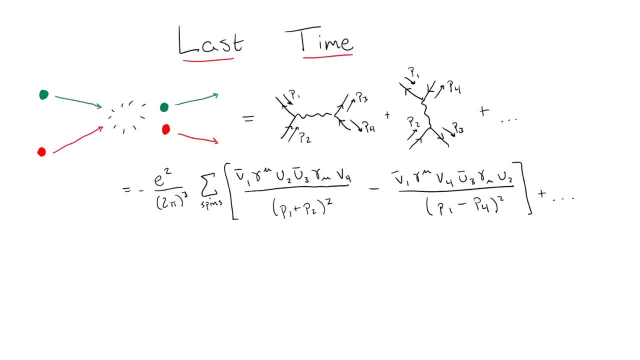 thing I didn't talk about is the somewhat disturbing habit that many of these perturbative calculations have of blowing up and becoming infinite. Some of these infinities are nothing to worry about, since they're cancelled off by considering other related processes. However, 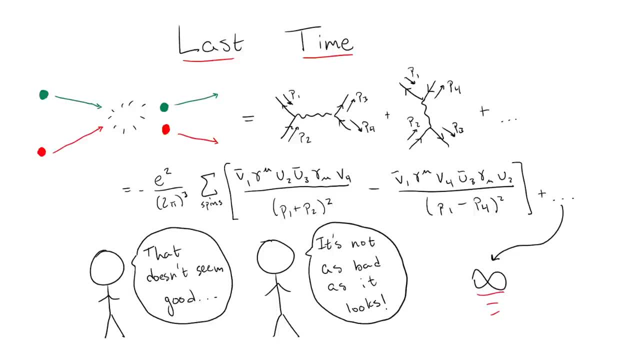 other divergences are still left over and seem to cause massive problems with our calculations. So how do we ever get meaningful calculations out of our theory when we seem to run into these problematic divergences at every corner? The answer is that we need to use a technique. 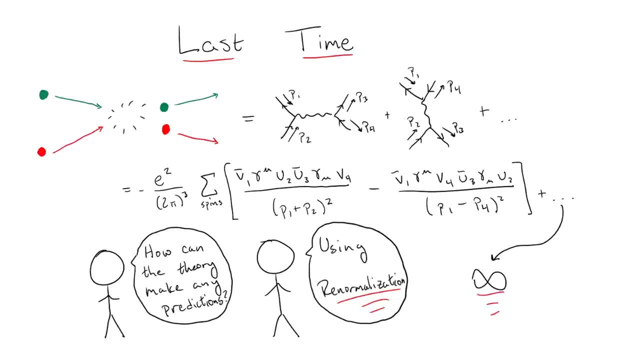 known as renormalization. Now, renormalization tends to be a bit of a touchy subject, Especially when people are first learning it, But hopefully by the end of this video I will convince you that it isn't really anything mystical or mysterious: It's a perfectly 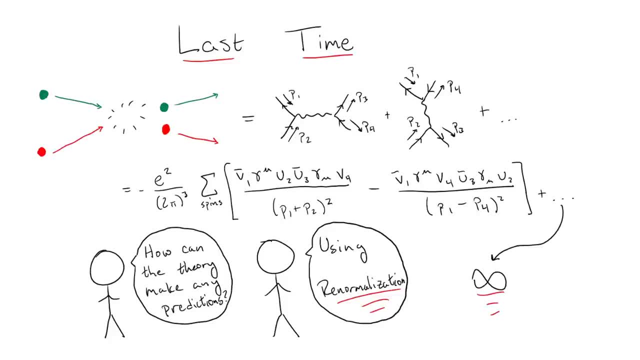 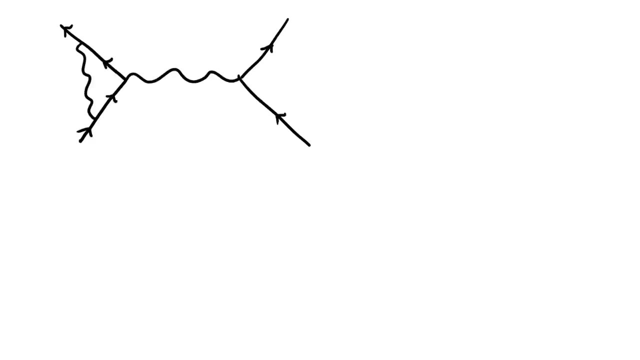 valid mathematical trick that we can use to extract meaningful results from our calculations that at first seem misbehaved. To begin the discussion, we should first understand where these divergences come from. To do that, we will use a somewhat simple example. Consider this Feynman diagram, which contributes to: 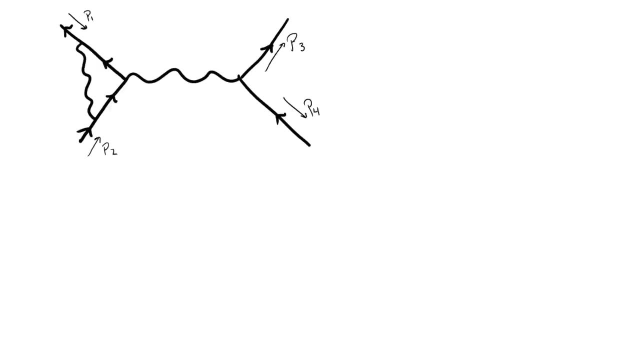 the fact that the number of divergences in this diagram is less than the number of divergences in the first order. This leads to the second-order correction to our QED-Baba scattering process that we looked at in the last video. Now remember that we have to conserve momentum. 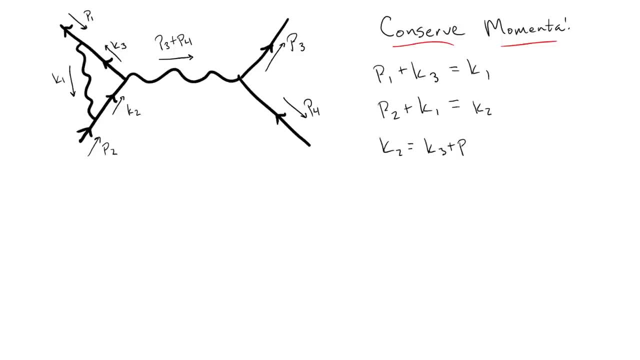 at every vertex of our Feynman diagram. When we work out the details of this momentum conservation, we find something interesting. Not all of the momenta of the internal lines are fixed. In fact, for every closed loop we have in a Feynman diagram, we get an extra unspecified. 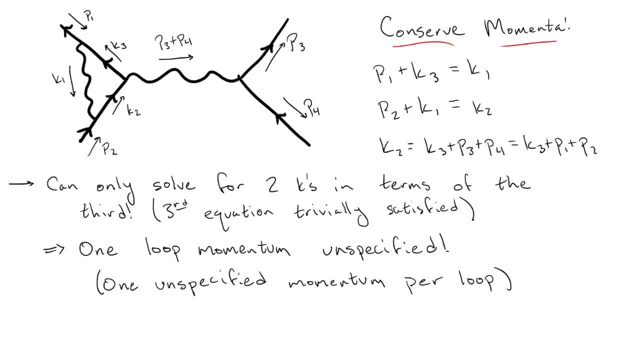 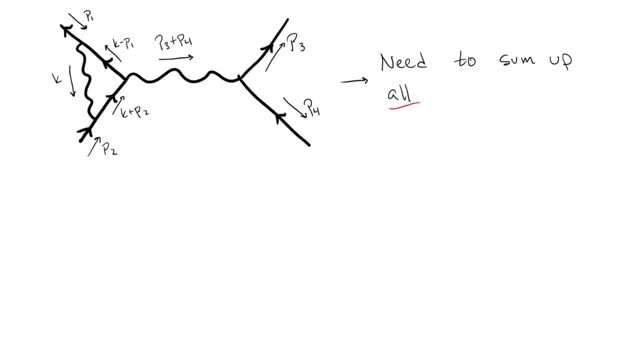 momentum. But since we have to add up all possibilities for the internal states of our Feynman diagrams, we have to sum or more specifically, integrate over all the possible values that this internal momentum can take. This integral is the source of our divergences. 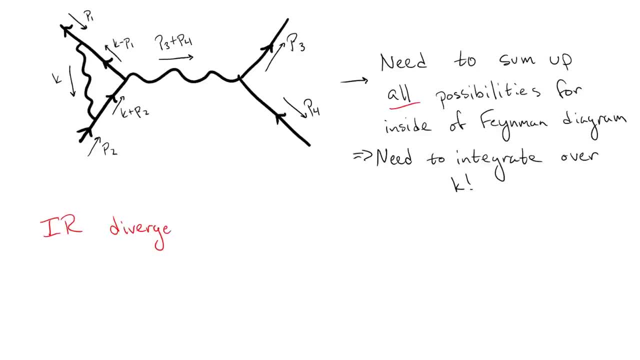 The region where the internal momentum goes to zero can result in low energy, also called infrared or IR divergences, while the region where the internal momentum gets very large can result in high energy, also known as ultraviolet or UV divergences. 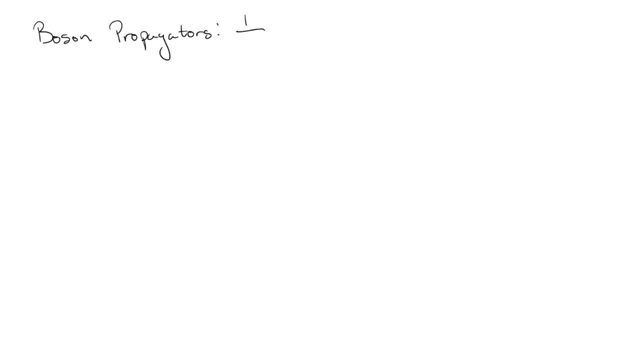 It should be noted that these divergences don't show up in every diagram that has a loop in it. IR divergences show up when we have massless particles in the loop. These are the divergences which end up cancelling with other effects like Bremsstrahlung radiation. 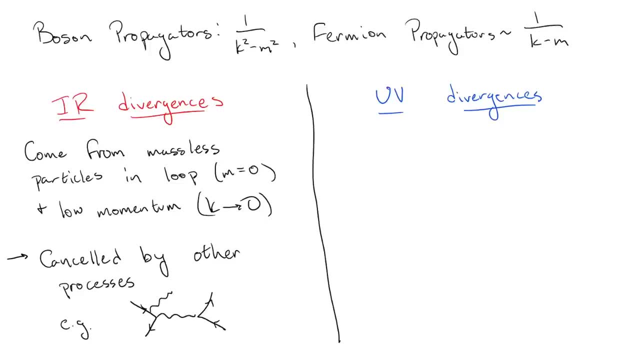 and aren't as worrisome, so we won't talk about these anymore. UV divergences, on the other hand, appear when there are only a few internal lines. This is most easily seen from the fact that each internal line is mathematically represented. 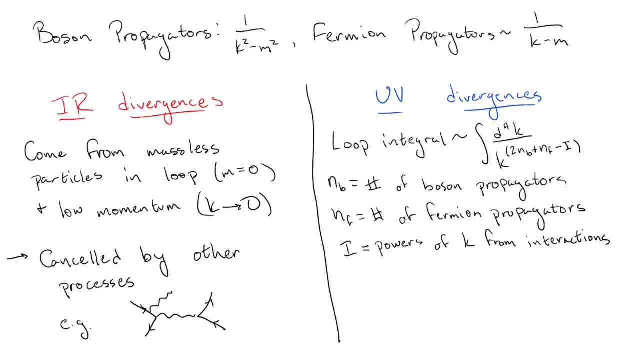 by a propagator, and the different propagators come with various powers of the loop momentum in the denominator. So if we have enough propagators, the integral for large momentum will actually converge and won't be a problem. Okay, now that we understand the source of these UV divergences we need to talk about. 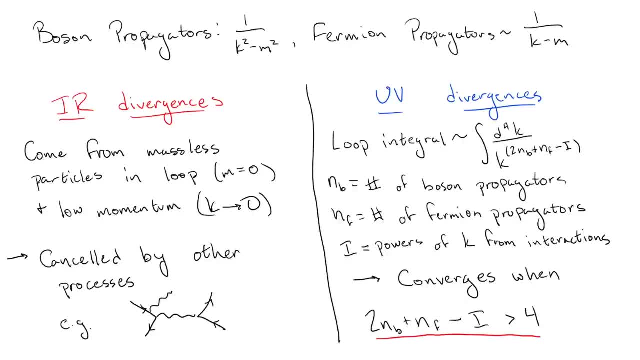 how to navigate them to make sense of our research. So let's get started To do this. we'll start with an analogy from the area of math known as singular perturbation theory. The example we will look at is a simple one. 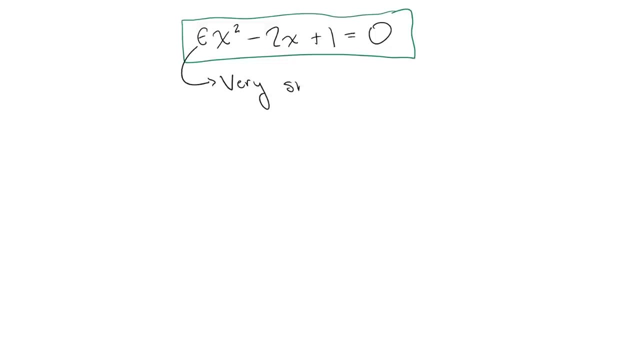 Consider this equation where epsilon is a number which we will assume to be very small. Now say we want to solve for x, but we have no knowledge of the quadratic equation so we can't solve it exactly. So we will find an approximation by perturbing an epsilon, or in other words, we write our 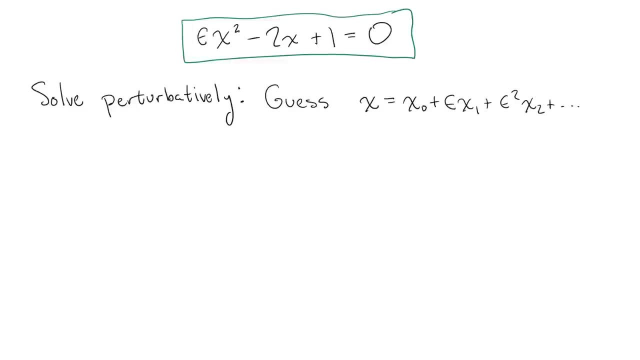 solution as a sum of terms with increasing power of epsilon. Now we just plug this expansion in for x in the original equation and separate our terms by the order of epsilon. Finally, we can solve this equation order by order in epsilon to find each term in our 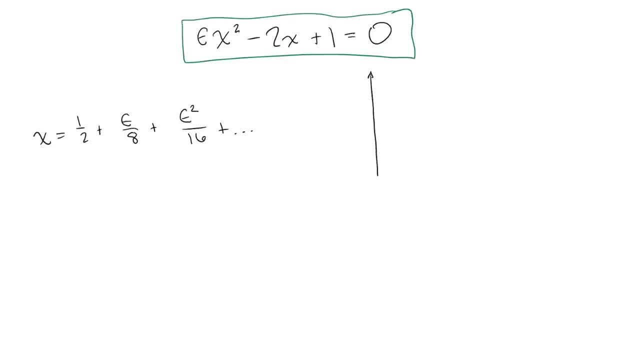 perturbative expansion. On the surface this seems fine, but if we try to plot this function, we will see that it actually has two roots, but we only found one. So what happened? Well, we can see that by keeping the epsilon in front of the x squared term in our function. 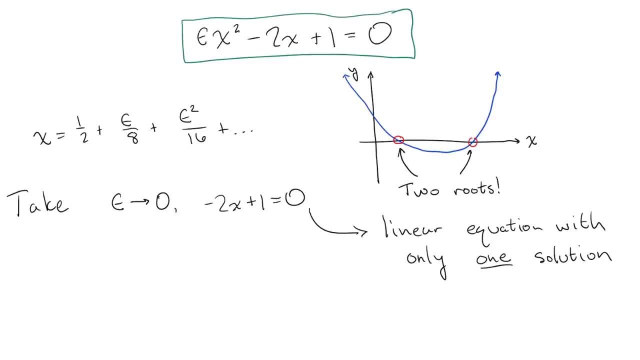 when we take the epsilon to zero limit in our perturbative expansion, we are changing the equation from a quadratic expression, which has two roots, to a linear one which only has one root. So we've found the one root of the linear expression, but we haven't found the second. 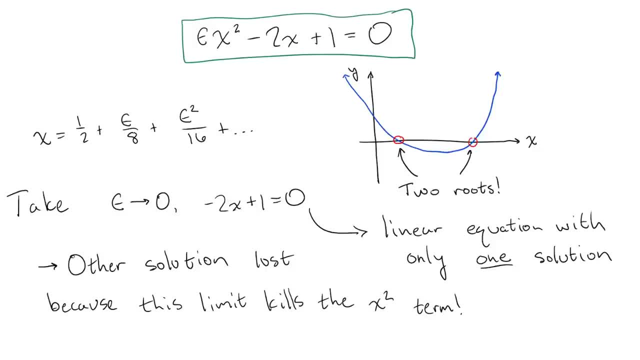 root from the quadratic expression. Obviously, something problematic is going on. So how do we find this other equation? Well, if we were able to somehow turn this expression into one which is still quadratic in the epsilon to zero limit, we could presumably recover the second root. 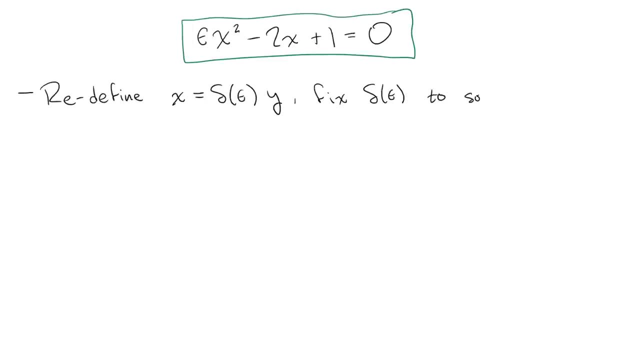 To do this, we will redefine our variable x to be, in terms of some arbitrary parameter, delta times y, which is the new variable we will solve for. Note that we have complete freedom to choose delta to be whatever we want, since any change. 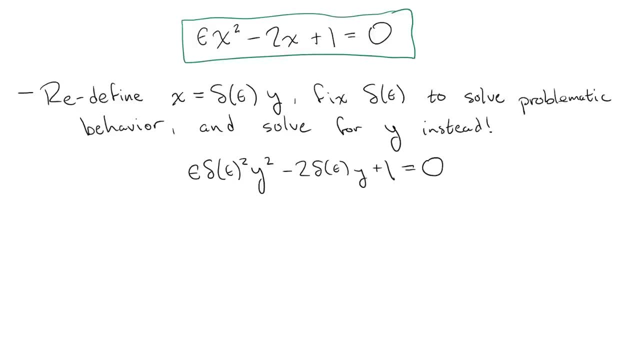 we make to delta will be compensated by delta times y. So we can now solve this equation. So we will define delta so that we both get rid of the epsilon in the y squared term, but also be careful not to introduce any extra 1 over epsilon terms, which might be an issue. 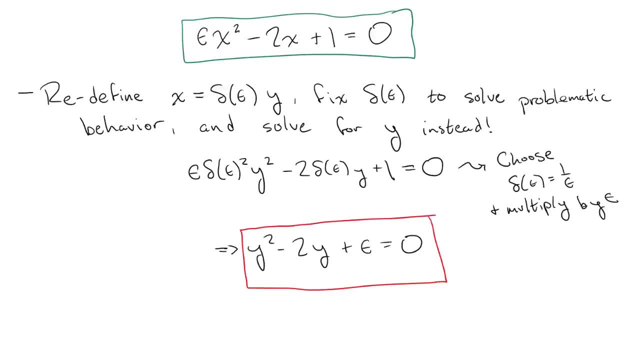 A good choice is just to make delta equal to 1 over epsilon, so that after multiplying the whole equation by epsilon we get a new equation for y that is still quadratic in the epsilon going to zero limit. Now we can write the solution for y as a perturbative expression. 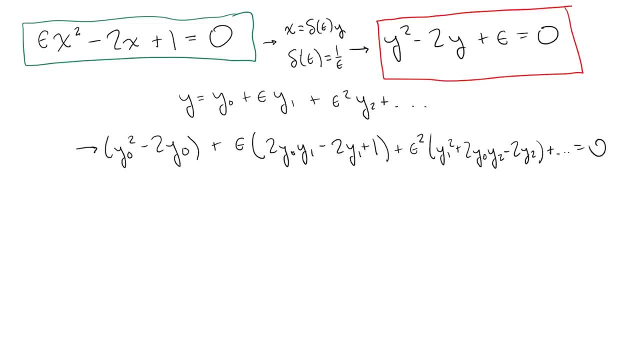 So we will define delta as the perturbative expression in epsilon and again solve order by order. When we do this, we amazingly recover our second root. Now, to find x, we just multiply these roots by delta and we have our perturbative solution. 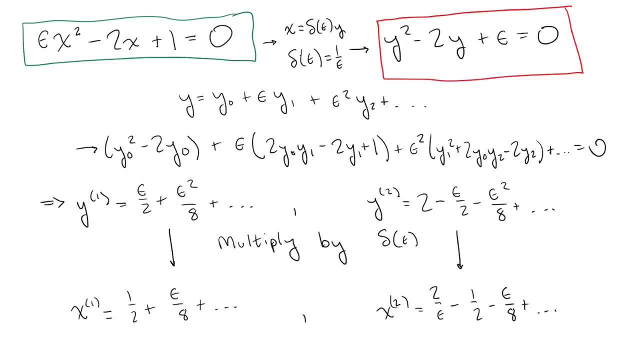 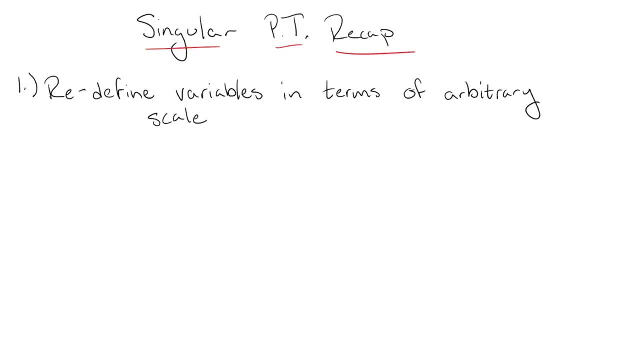 So we were able to get around the problematic behavior of the solution by using the following strategy. First, we redefine our parameters in terms of arbitrary scale parameters, delta in this example. Second, we choose by hand the scale parameters in order to artificially eliminate the problematic. 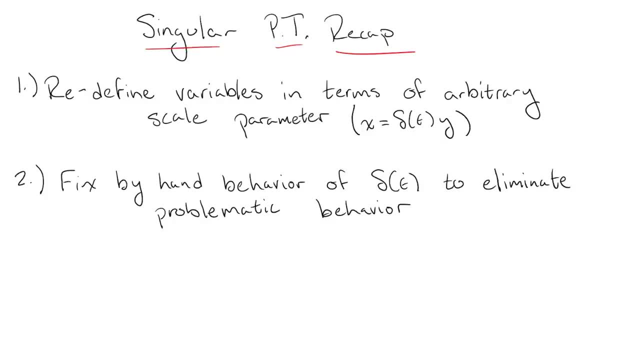 behavior in our equation so that we can actually solve the now well-behaved equations. Finally, we need to factor back in the scale parameters to get our true solution. One last thing before we move on to talking explicitly about renormalization in particle. 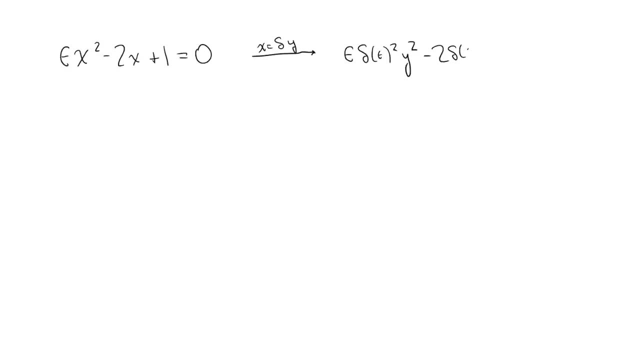 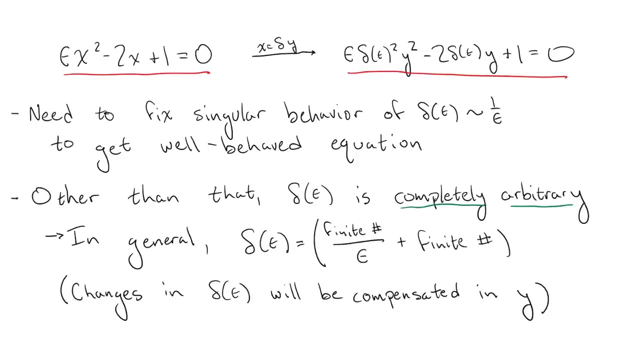 physics. Notice that our decision for the epsilon dependence of delta was necessary in order to remove the singular behavior from the equation we wanted to solve. However, since delta is otherwise arbitrary, we could also include any finite factors we want in delta. So say, we introduce a new parameter into delta, call it a, so that delta is a function of. 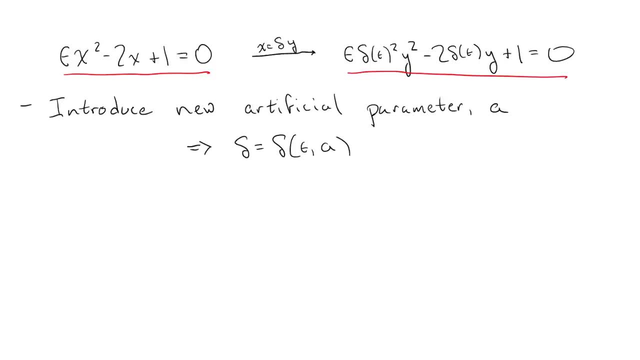 both epsilon and a, Then presumably a will show up in our solution for y as well. However, since we put this parameter in by hand and it doesn't actually exist in our original problem, X needs to be completely independent of a, meaning that when we multiply y and delta, 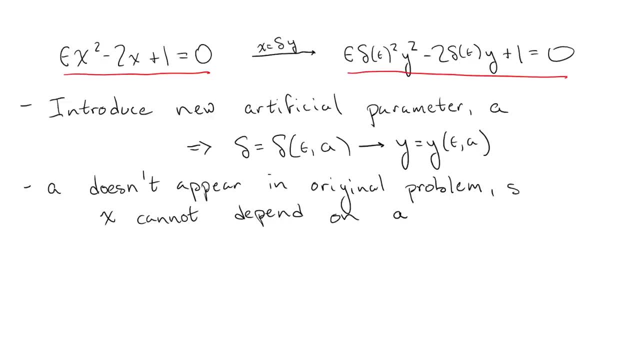 to find x. the a dependence in y should exactly cancel the a dependence in delta. In fact, we can even write down a differential equation which encapsulates this. Now, since a can never show up in our solution of x, this equation should be satisfied at: 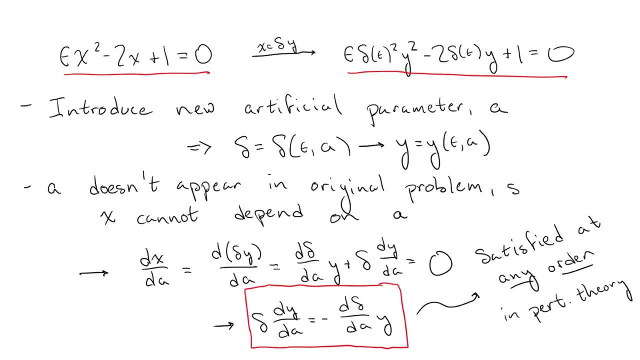 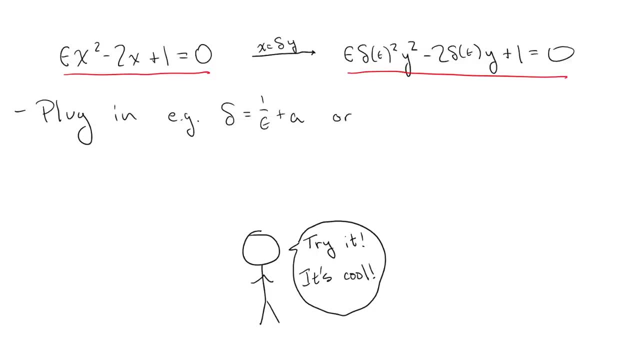 every order in perturbation theory as well as overall. This is actually something that I encourage you to try. Just do the same thing we did before, but add in any finite term. you want to delta and solve the perturbative expansion for y in exactly the same way. 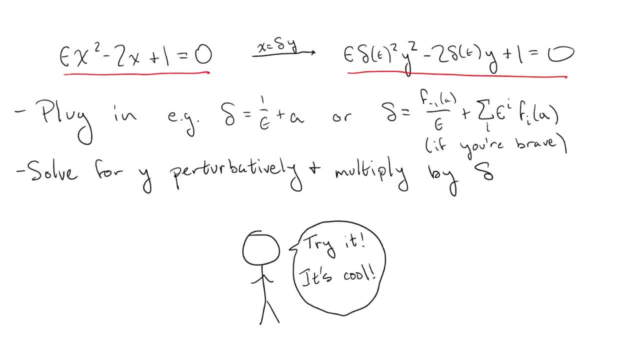 You'll see that almost magically, order by order, in perturbation theory these finite terms exactly drop out to give the same answer for x that we found before. Of course it isn't magic, because this must be the case for everything to be mathematically. 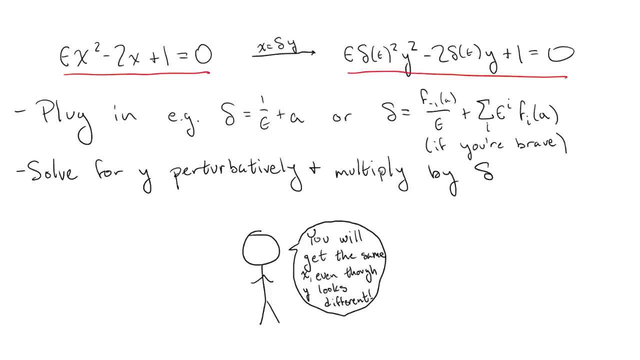 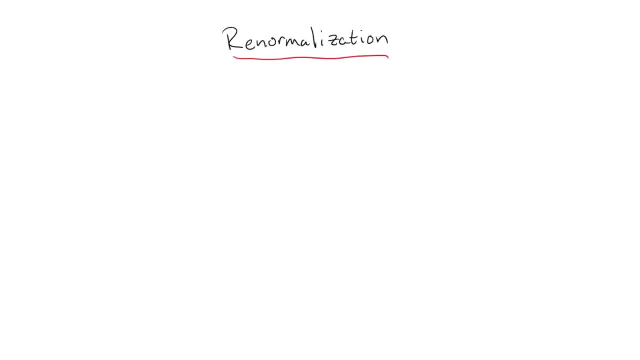 consistent. Okay, so what does all of this have to do with renormality? Well, it turns out that this whole discussion is almost exactly the same as what we do when we renormalize a theory in particle physics. See, in our theories we have a certain number of parameters which are not fixed by the theory. 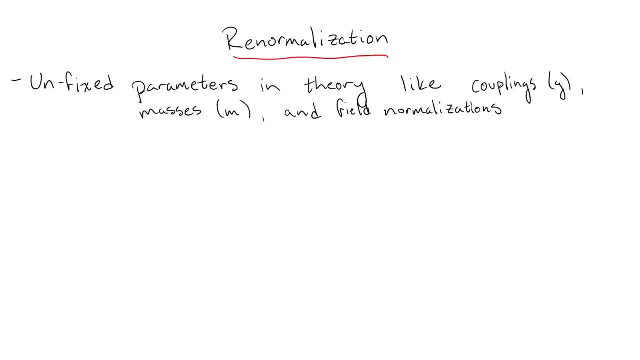 itself. These tend to be things like coupling constants between fields, masses of particles and field normalizations. So, just like we did for x a minute ago, we can rescale these by some arbitrary method. So what we're going to do now is we're going to do the same thing over and over again. 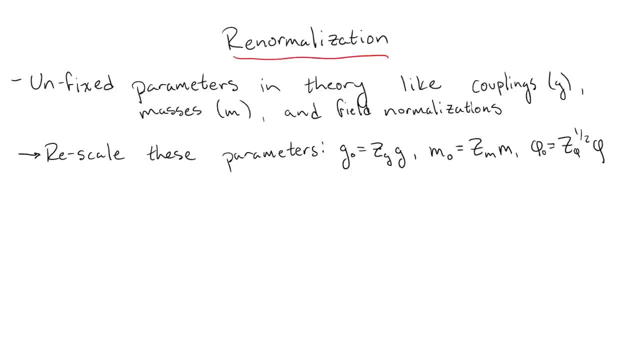 We are going to say this first. Now let's think about the basic definition of a function and what this is all about. So what we're going to do is we're going to say, if a function of this value is fixed by a number of variables, that this component of the variable is fixed by a function of. 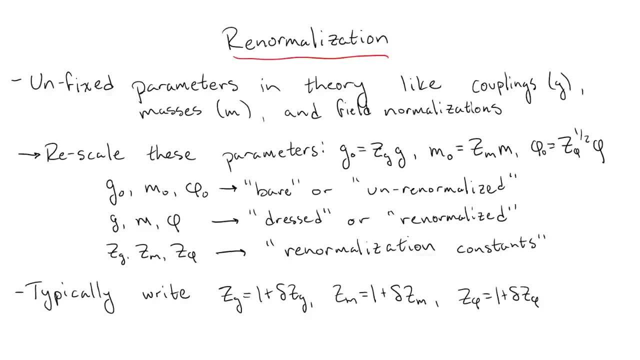 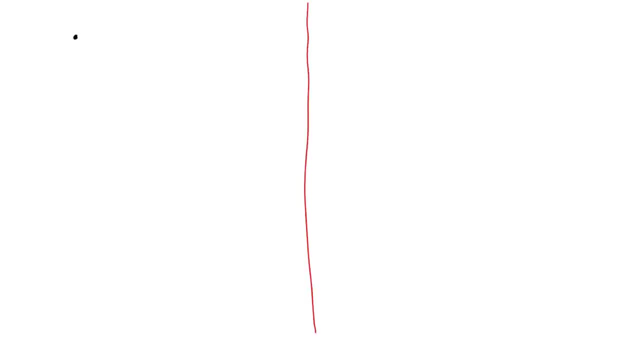 x, then we're going to write the function of the variable x. Now, what this function of x is really going to do is that it will, in the same way we, the Feynman rules from our original theory, but with the bare parameters replaced by their 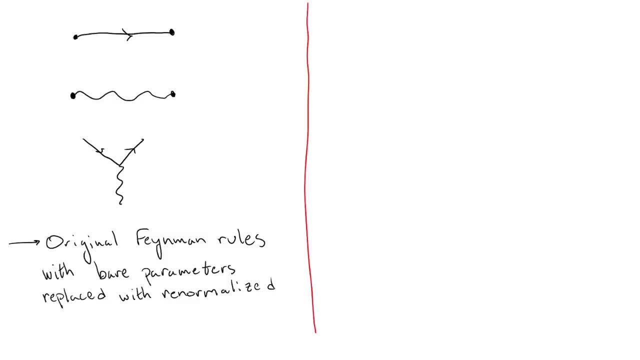 renormalized counterparts. However, it also has an additional consequence of adding in a new set of Feynman rules that we didn't have before. These Feynman rules all come with factors of counterterms, and we will denote them by including an x inside the diagram. Now remember, this is all. 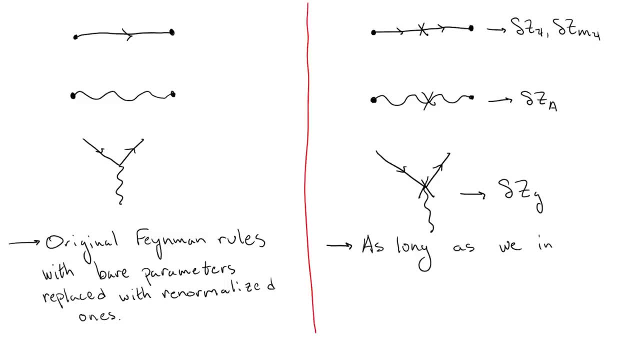 still completely artificial. This is exactly the same theory that we had before. we've just shuffled things around to make it look slightly different. As long as we include all possible Feynman diagrams, including ones with these new counterterm vertices, we should get exactly the 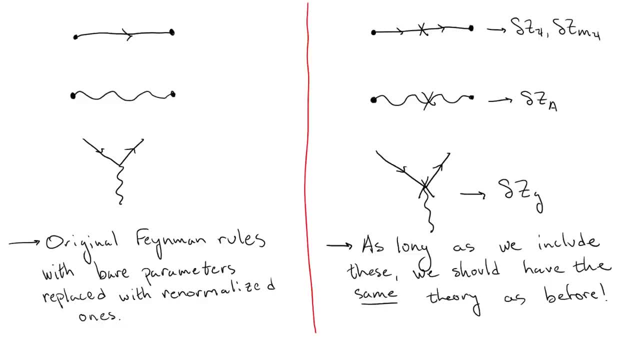 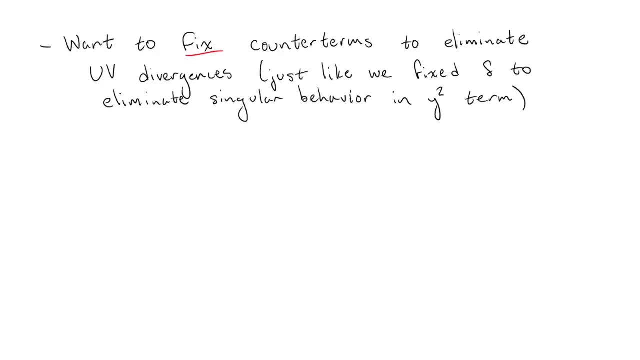 same answer as we would get in our original theory, just like how before we recovered x by multiplying y by delta. So now we need to fix these counterterms. We want to choose them to eliminate the problematic UV divergences which show up in the theory, just like how we chose. 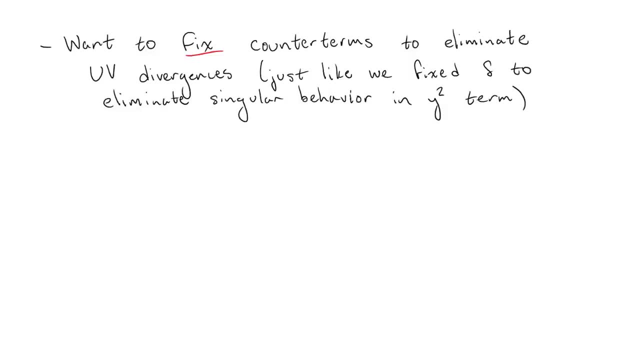 delta to eliminate the dangerous leading order behavior of our quadratic equation. But how exactly do we do that? Well, these new Feynman diagrams with counterterms in them correspond to a certain set of external states which we can reproduce using Feynman diagrams without counterterm. 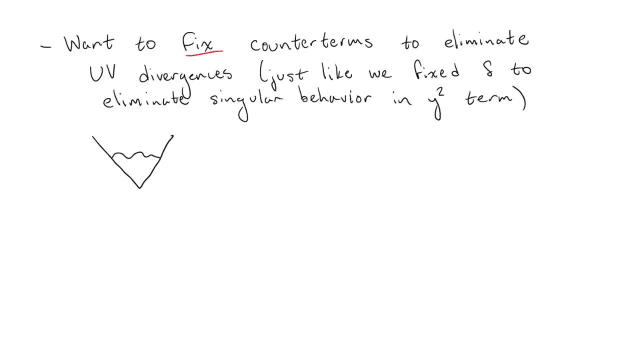 insertions. For example, if we look at loop corrections to the QED vertex now using the x and y-axis, we can see that the x-axis is the same as the y-axis of the x-axis. of the x-axis, Using the renormalized parameters, these have the same external state as the counterterm diagram. 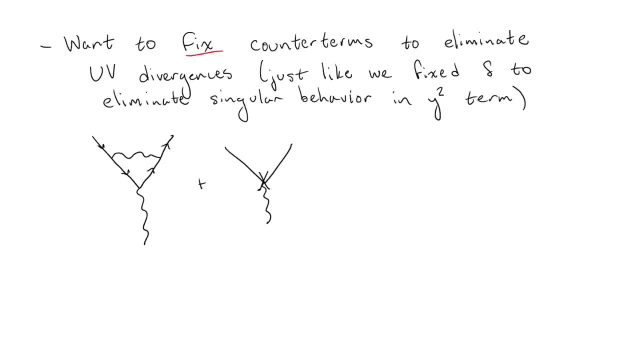 which includes a factor of the coupling counterterm. The loop corrections can be UV divergent for the same reason as before. So if we define the counterterm so that it exactly cancels these divergences, the corrections to the QED vertex will always be finite. 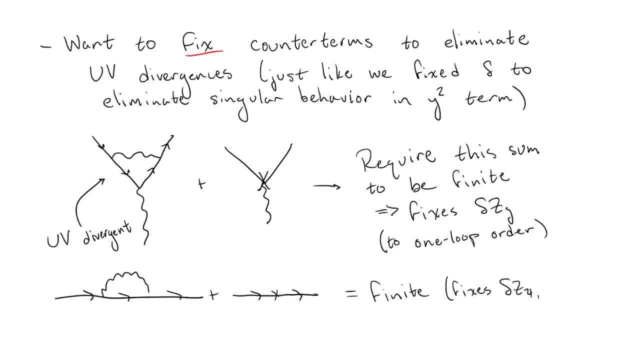 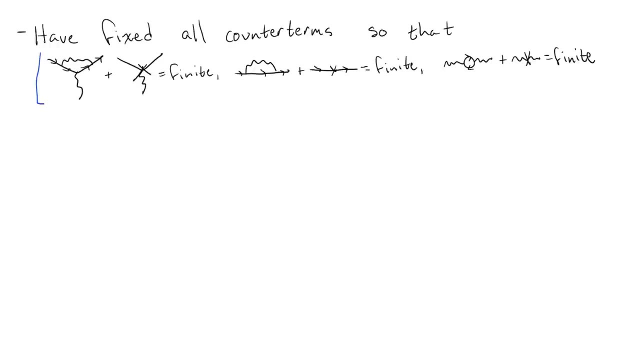 We can also do this same procedure with loop corrections to the propagators to find the counterterms corresponding to our fields and our masses. So at this point we've completely fixed the divergent behavior of our counterterms so that they cancel specific divergences in our theory. 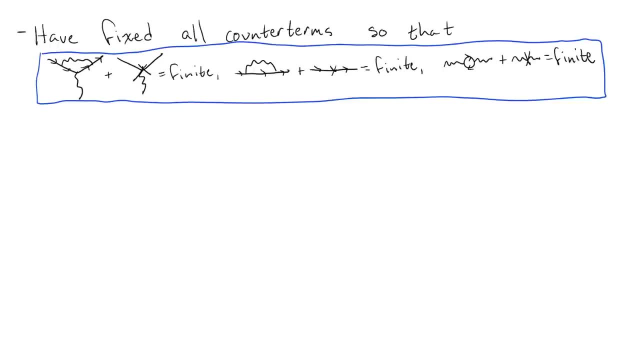 Now we can return to our example of ba-ba scattering. We can do the calculation in exactly the same way we did before, except now use renormalized parameters instead of the bare parameters, But this doesn't give us the full result, As we just. 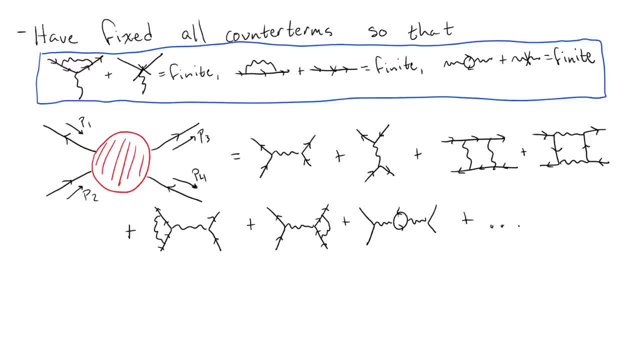 As we just said, to recover the full result, we need to also include all of the diagrams which come with counterterm insertions as well, up to a given order, and perturbation theory. In this simple example, it's easy to see what will happen. 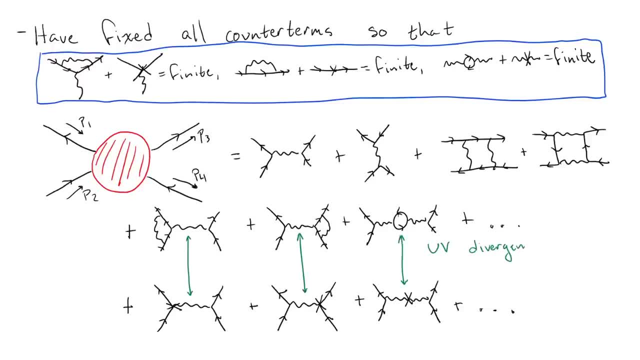 We'll be able to pair up divergent diagrams with corresponding diagrams with counterterm insertions and when we add them together, the sum will end up being finite due to the way that we chose to define our counterterms. At the end of the day, we will have a completely finite calculation of the amplitude for electron-positron. 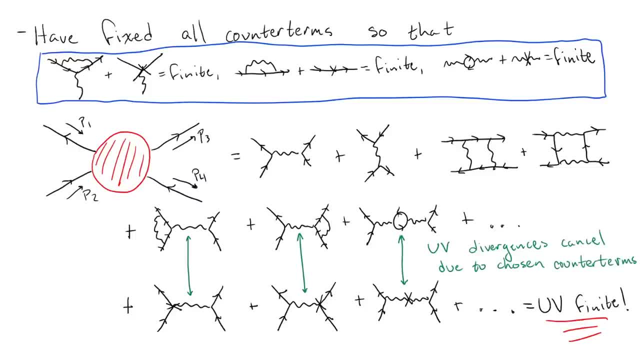 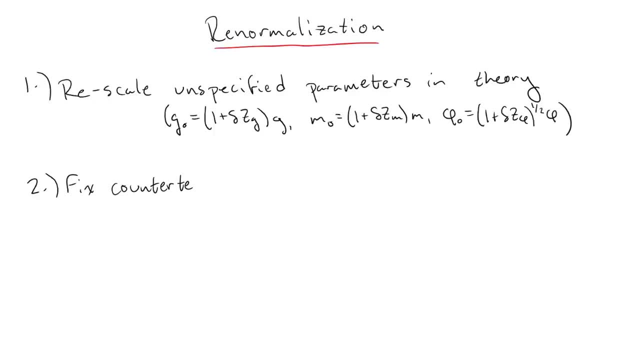 scattering Again. we haven't done anything wild or magical. We simply rescaled parameters which are not determined by our theory, chose these scale factors in a convenient way and took the rescaling into account in a consistent way later on, by including these counterterm Feynman rules in our perturbative expansion. 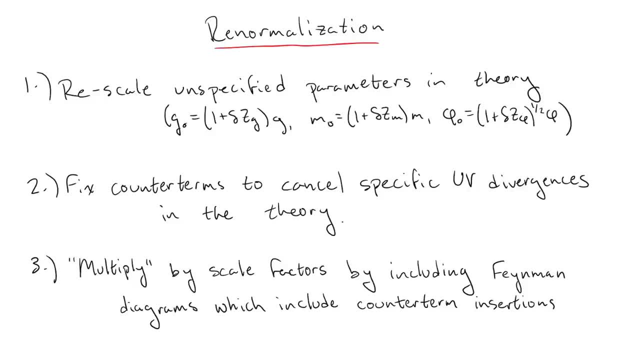 At higher orders. in perturbation theory, the details get a bit more complex, But the general story stays the same. Ok, so now we've seen how renormalization can be used to render all of our amplitudes finite. This is amazing, but it still isn't the end of the story. 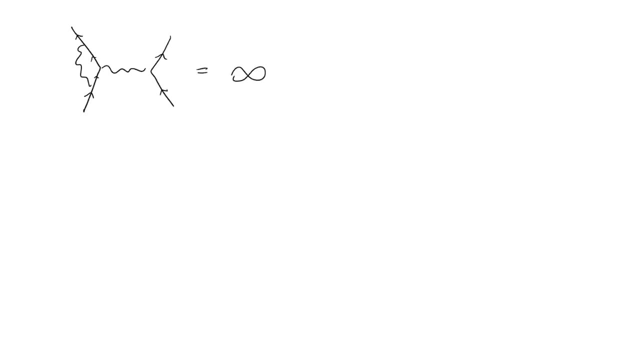 When we're trying to calculate these divergent integrals, we can't just plug in infinity, since this will completely wash out all of the finite behaviors that we actually care about. So we have to regulate the integrals somehow. We almost have to do it all over again. 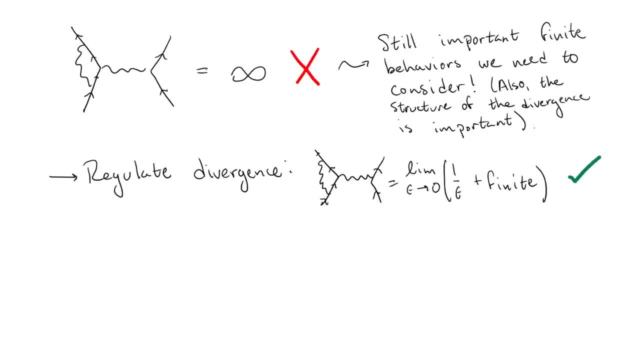 them to give a finite result and then take a limit at the end of the calculation. This can be done in many different ways, but two of the most common are to simply impose a maximum value that the loop momentum can take, known as a momentum cutoff scale, and eventually take the limit as 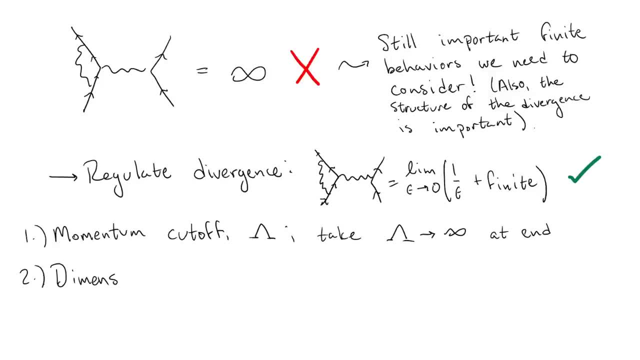 this cutoff scale goes to infinity. Or we can work in an arbitrary number of dimensions, known as dimensional regularization, and take the limit as the number of dimensions goes to four. In both of these methods of regularization one must introduce an artificial energy scale In the momentum cutoff. 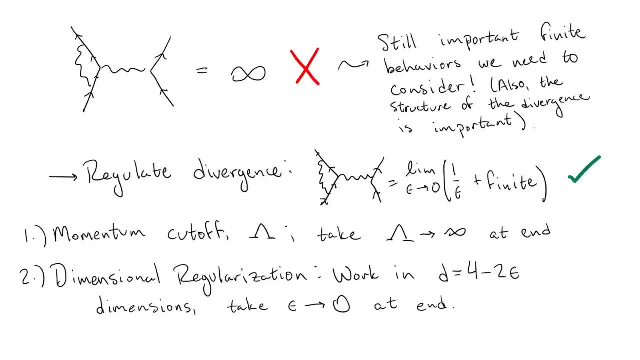 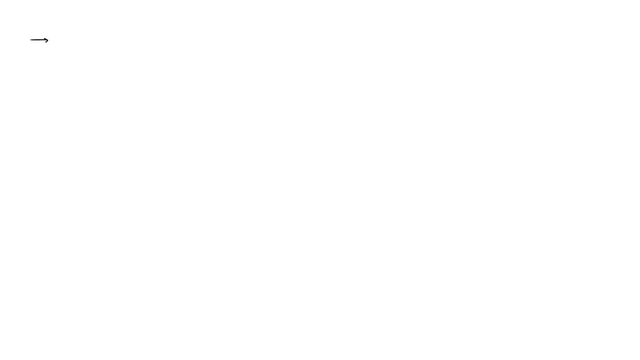 case, this energy scale is the cutoff itself, While in dimensional regularization, it's a little more complicated to see how this scale arises. Regardless of how the energy scale arises, it's something that we have to insert by hand in order to find the right value for the loop momentum. 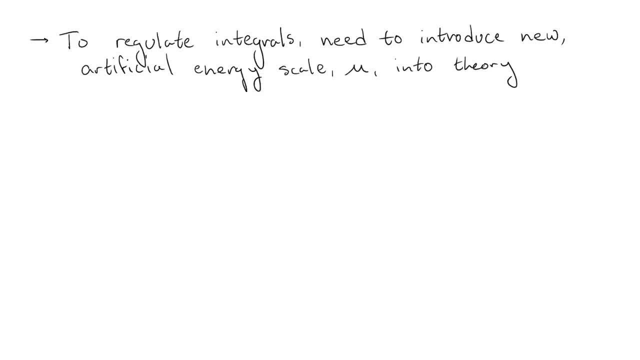 Since it doesn't show up in our original theory, our bare parameters must be completely independent of this energy scale, exactly the same way that, if we choose to include any new parameters into delta and y that didn't show up in our original quadratic expression, x could not depend on these. 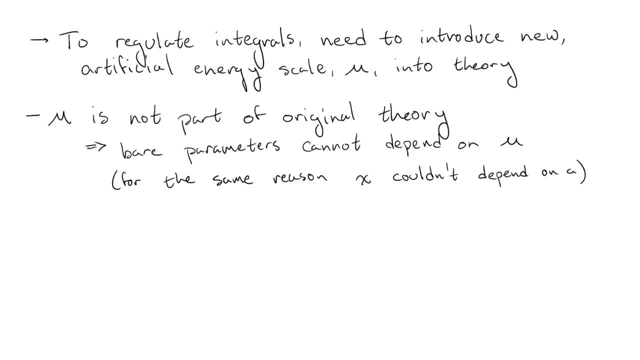 parameters In an exactly analogous way as before. this gives us a set of differential equations relating the dependence on the new energy scale of the renormalized parameters to that of the renormalization constants. This set of differential equations is known as the renormalization group. 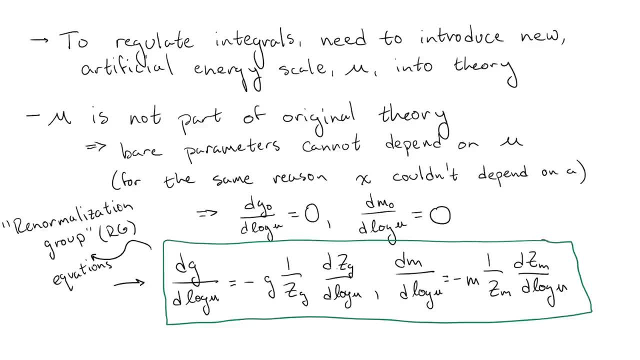 equations, or RG equations for short. The RG equations guarantee that physical observables are completely independent of this energy scale, even though it shows up in intermediate calculations. One result of this is that we find that the renormalization of the energy scale is not 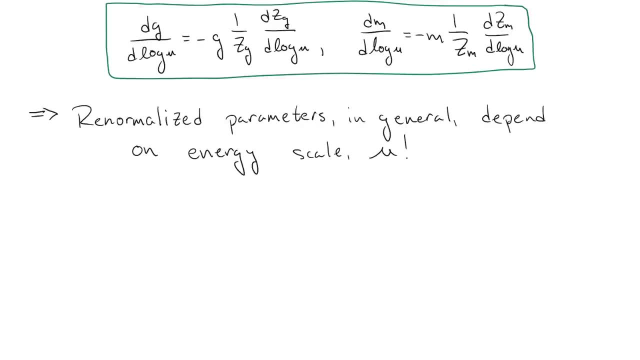 only the差不多 of some energy scale, but also that it applies to all Houston and this data is actually dependent on the energy scale that we choose. So here we have to be careful. We are doing perturbation theory in the power of the renormalized. 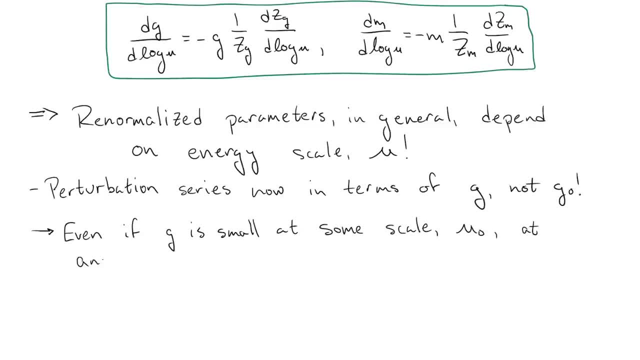 couplings, which means that we assume that these couplings are small. If these couplings can change with energy scale, there's a chance that they will at some point become large enough for perturbation theory to break down completely, meaning that: 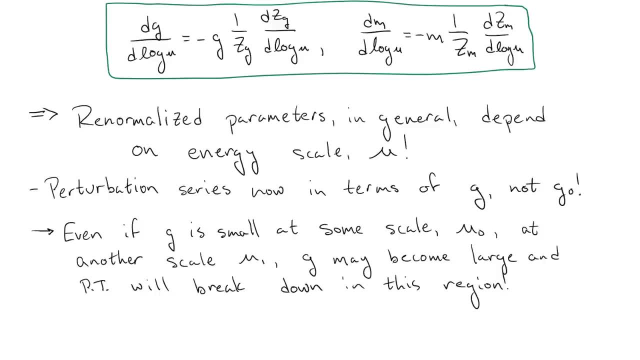 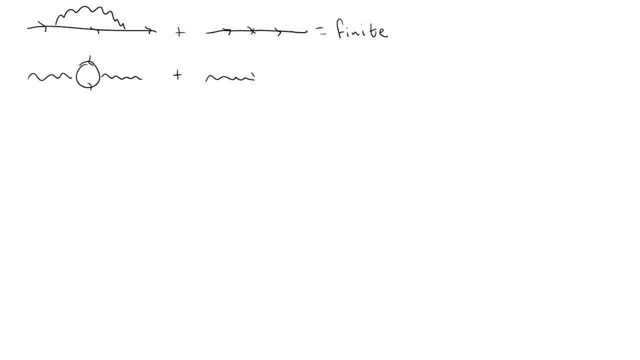 our intermediate calculations, before this artificial scale drops out will be fractions out are invalid. This actually happens in the standard model with quantum chromodynamics at low energies and is one of the reasons why hedronic calculations are so difficult to compute. In addition to this, we can of course add in any finite terms we want into our counterterms. 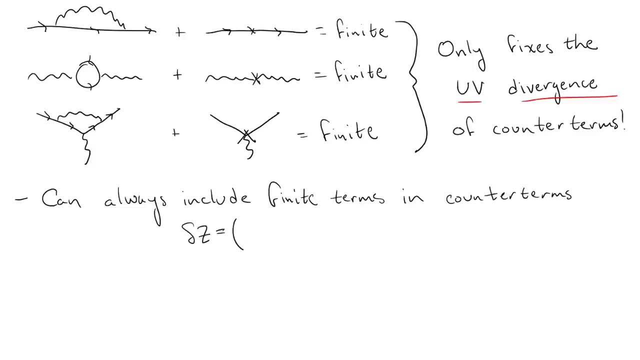 as long as we compensate for it in the renormalized parameters. This choice is known as a choice of renormalization scheme. The two most common choices of renormalization scheme are: to not include any finite terms known as the minimal subtraction, ms or ms-bar scheme. 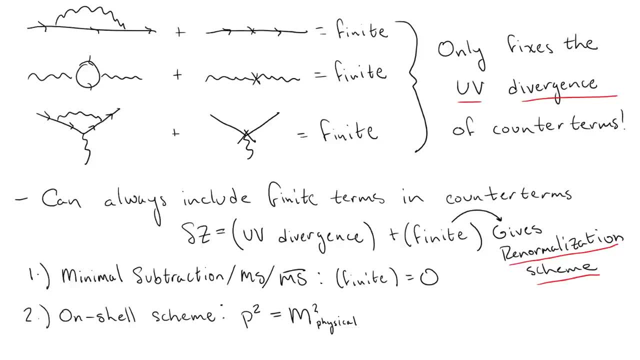 or to fix everything so that on-shell particles always have the masses which are measured by experiments known as the on-shell scheme. Again, at the end of the day, our final calculations should be completely independent of our choice of scheme, so we can't do anything about it. 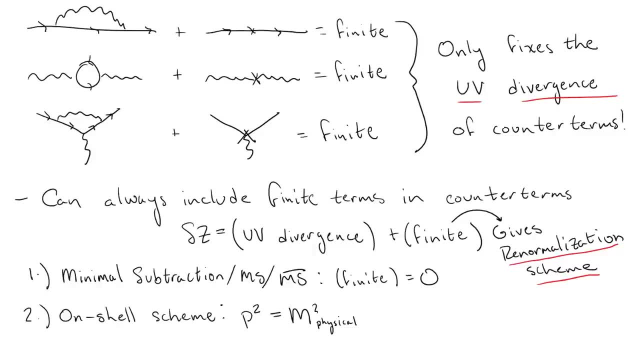 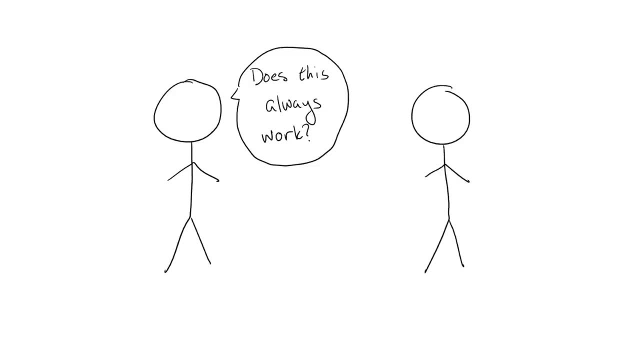 We can choose whatever is best suited for the calculation at hand. Now I'm sure that many of you are also asking: does this actually work? in general, Are we guaranteed to always have all of our divergences drop out if we do the renormalization correctly? 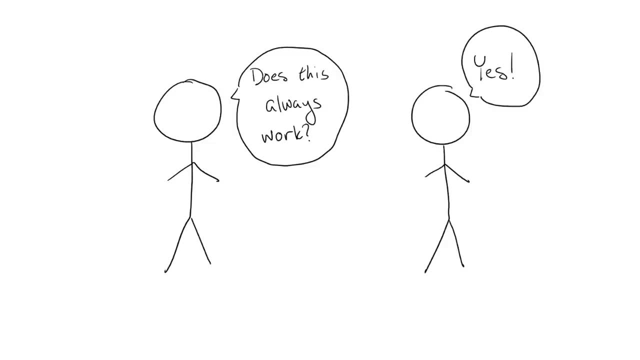 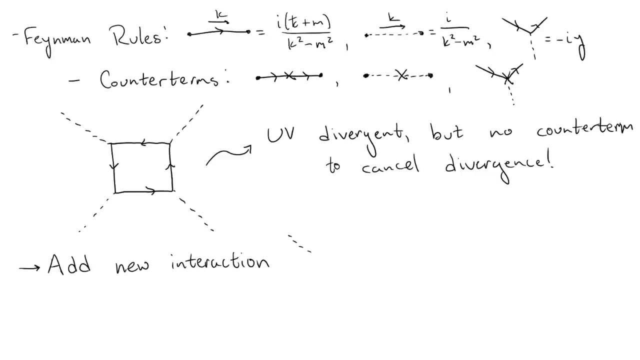 And the answer, surprisingly, is yes. The reason why is actually fairly simple to see. Say, we have a diagram with a certain set of external states whose divergences are not cancelled by the counterterms we have. All we have to do is include a new fundamental interaction with this set of external states in 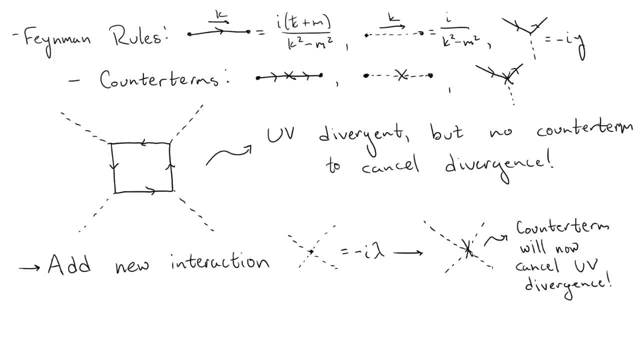 our theory, This new interaction will have a corresponding coupling, which of course gets its own counterterm, which we can use to cancel this leftover divergence. This may seem completely unacceptable at first, but think of it this way: We're doing perturbation theory in terms of 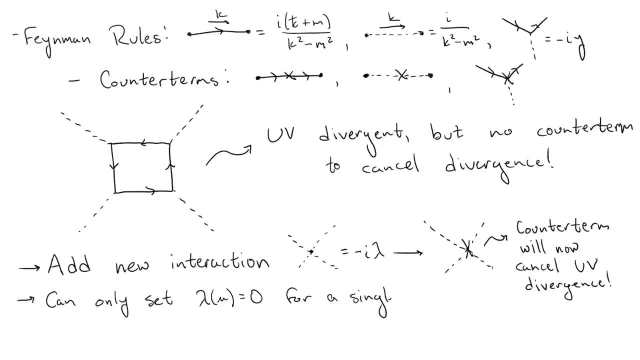 renormalized couplings, and we've already seen that these pick up an energy dependence. If we try to not include one of these interactions in our theory, this just corresponds to setting the coupling to zero, But we can only really set it to zero at a given energy scale, in which case at any other, 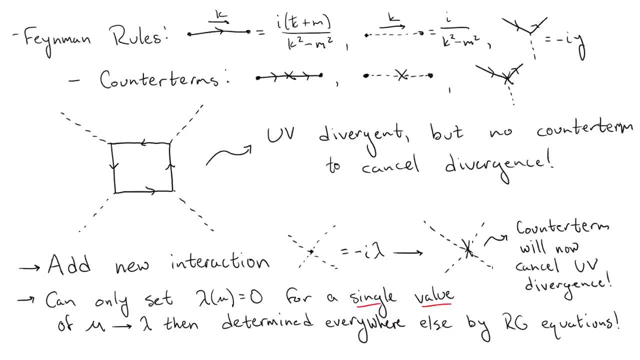 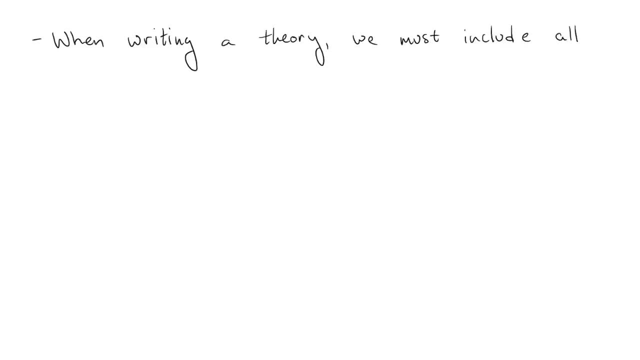 energy scale, the coupling will run to a different value and we will generate this new interaction. This tells us that we have to include all of the interactions in our theory whose counterterms cancel ultraviolet divergences. This will automatically split our theory and we'll have to. 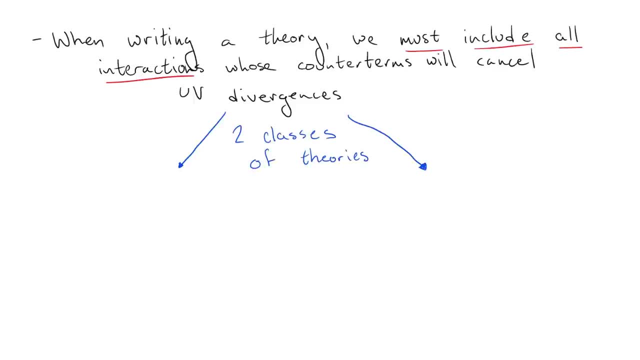 divide it into two classes: Those where we only need a finite number of interactions to cancel all divergences, and those where we need an infinite number of interactions. The names of these classes of theories are a bit unfortunate. The former are known as renormalizable theories. 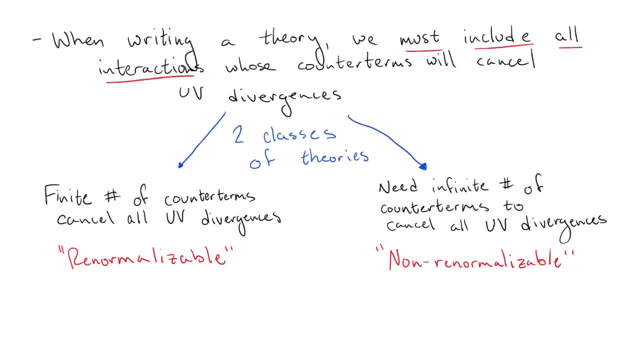 while the latter are known as non-renormalizable. However, non-renormalizable is a bit of a misnomer. Nothing really breaks down when we apply a renormalization technique. it just turns out that we'll need an infinite number of terms in our theory. 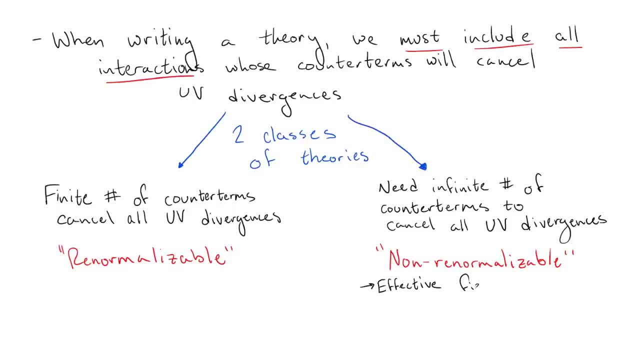 The non-renormalizable theories also have a very nice interpretation as effective theories, approximate theories which work very well, but only up to a given energy scale. As a great example, if we try to quantize general relativity, we end up with a non-renormalizable 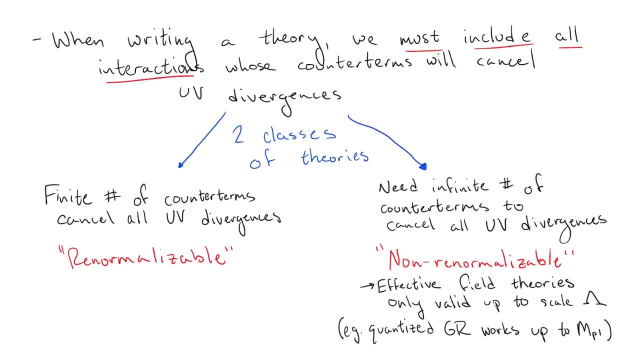 theory. This means that we can still do approximate perturbative quantum gravity calculations, but these calculations will not be as effective as they used to be. The non-renormalizable theories are known as perturbative quantum field theory calculations. The non-renormalizable theories are known as perturbative quantum field theory calculations. 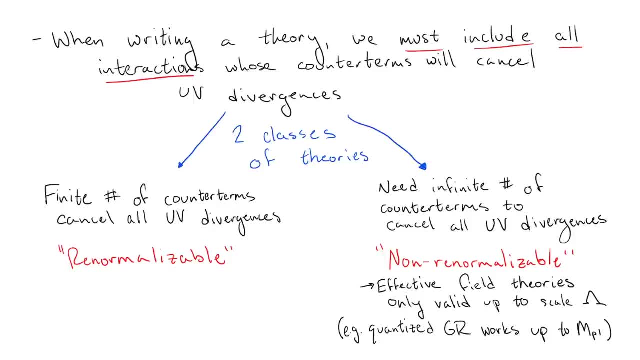 but these calculations break down at a high energy scale, namely the Planck scale. This just means that if we try to look above this energy scale, we should expect to see some new physics appearing which can be described by a more fundamental quantum description of gravity. 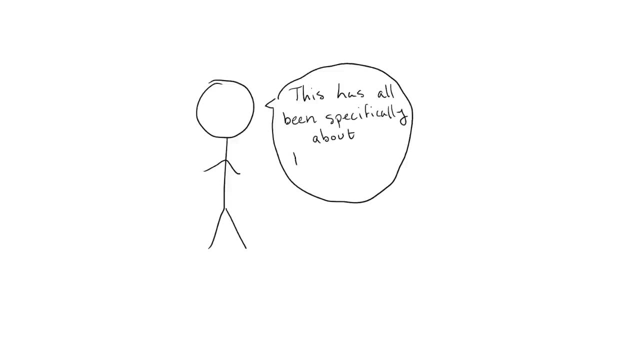 As one final note, everything that I've talked about here is specifically known as perturbative renormalization and is usually what's used in particle physics or perturbative quantum field calculations. There are other contexts where renormalization shows up, such as in statistical physics and 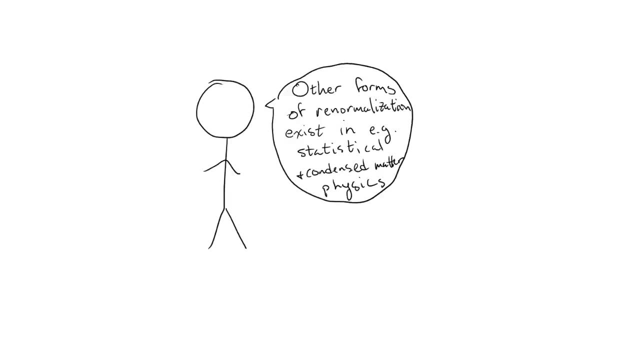 condensed matter systems where the discussion is somewhat different but still shares similarities, such as problematic behaviors arising with short-distance or high momentum effects and the importance of being able to compare the theory at different energy scales. If you've made it this far in the video, hopefully I've been able to convince you. 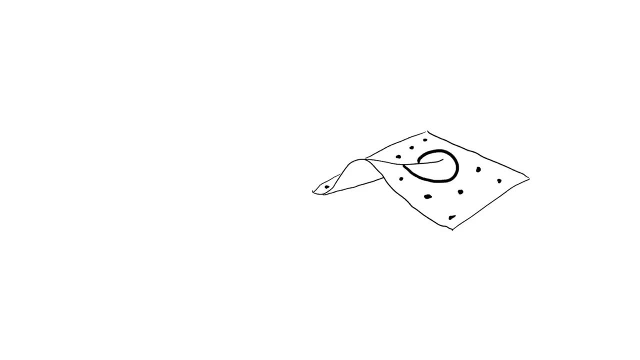 that renormalization is not somewhat the number one theory, wild thing that particle physicists use to sweep infinities under the rug. Instead, it is just a reshuffling of parameters in the theory, which allows us to explicitly treat the theory where a naive treatment fails, On top of allowing us to actually do calculations in the first place.